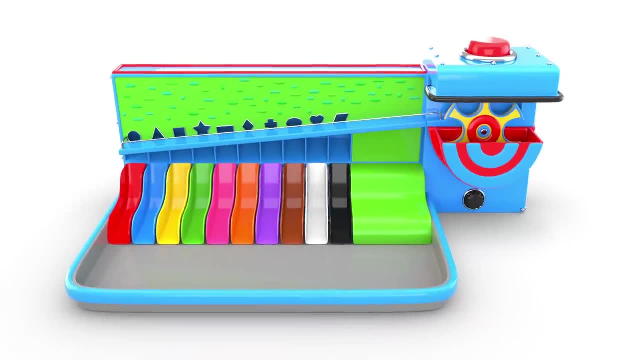 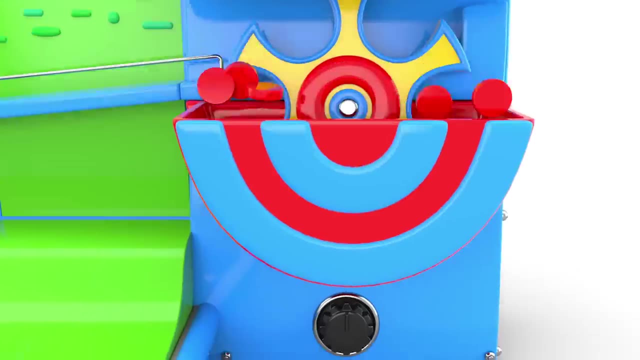 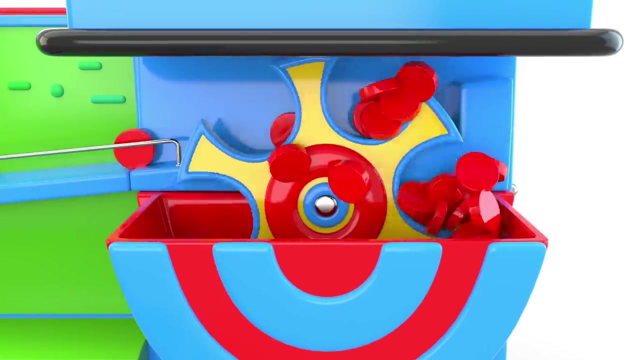 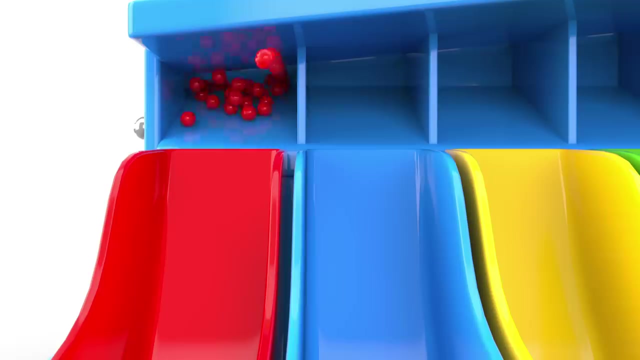 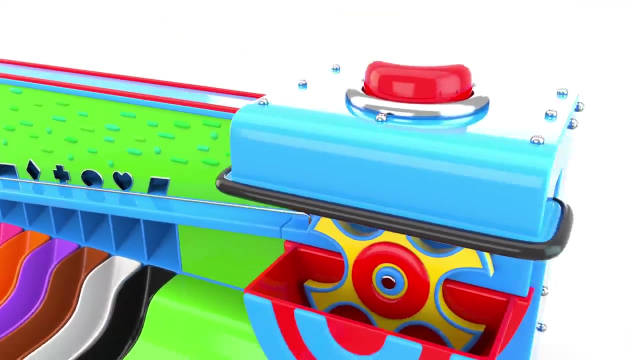 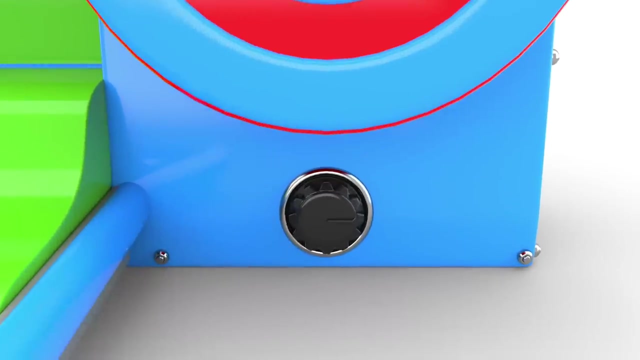 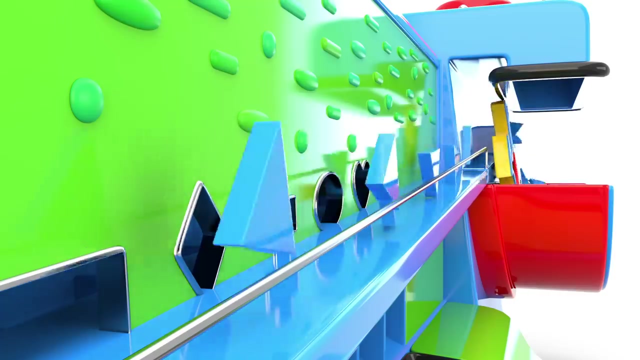 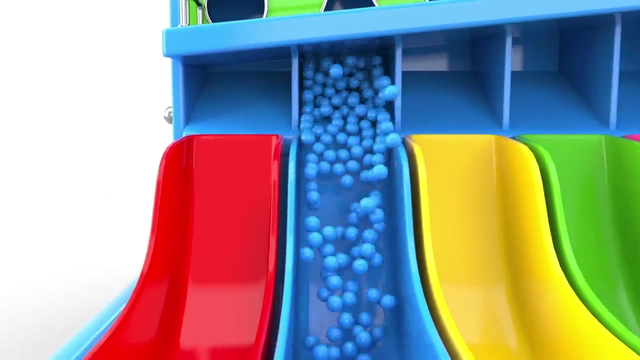 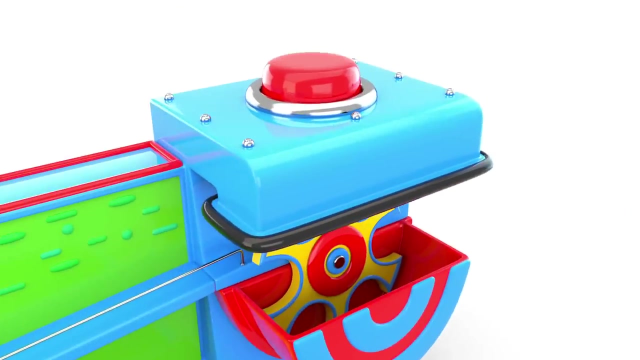 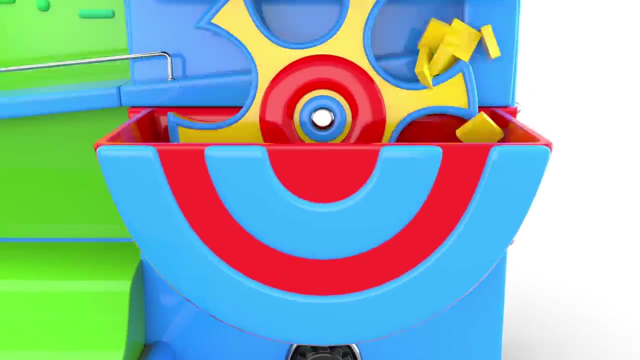 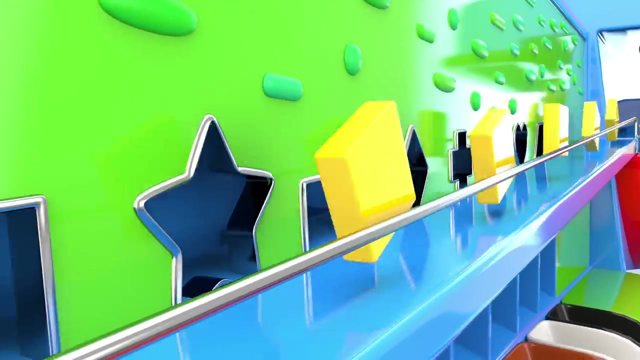 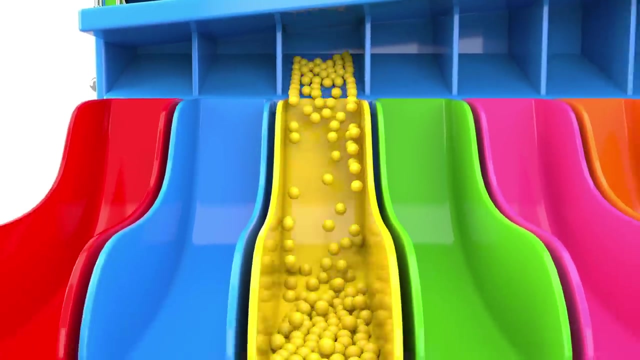 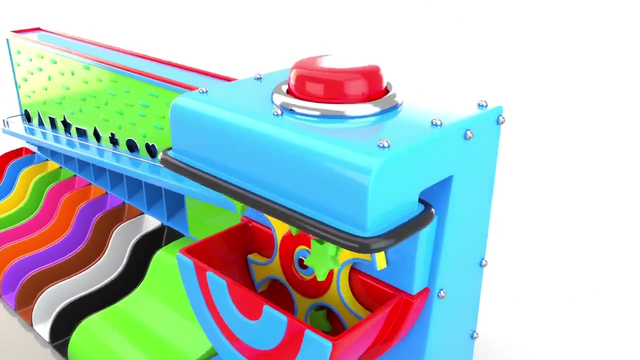 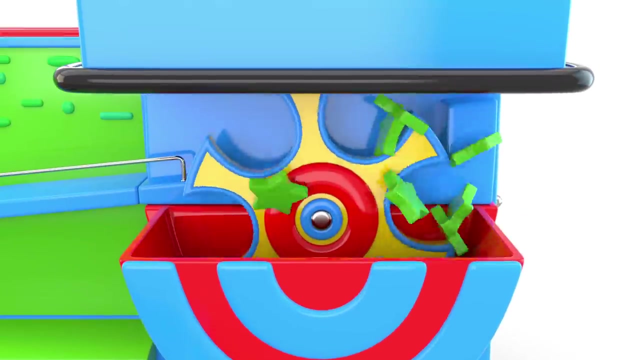 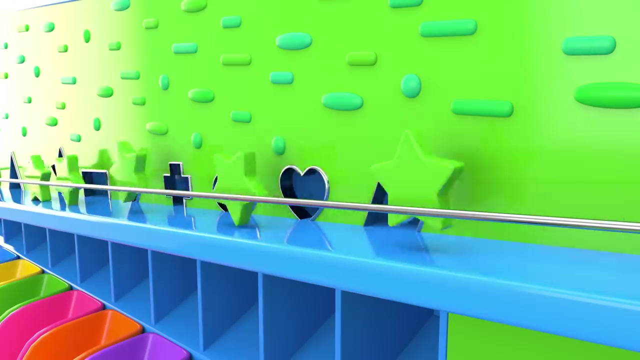 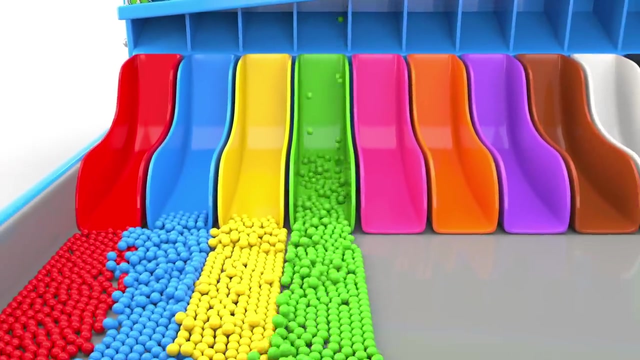 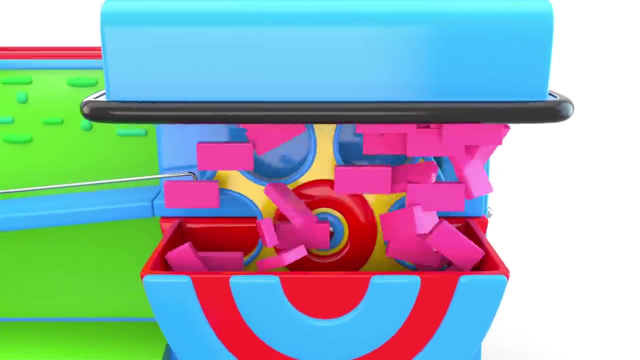 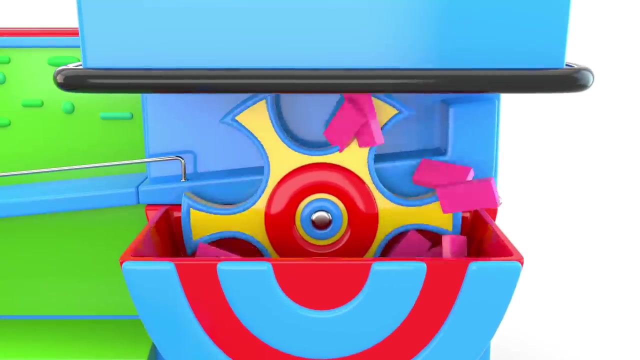 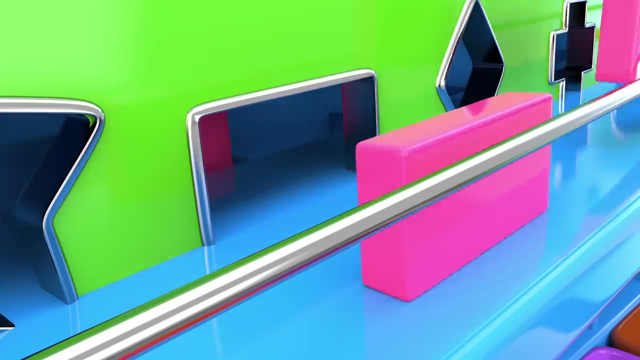 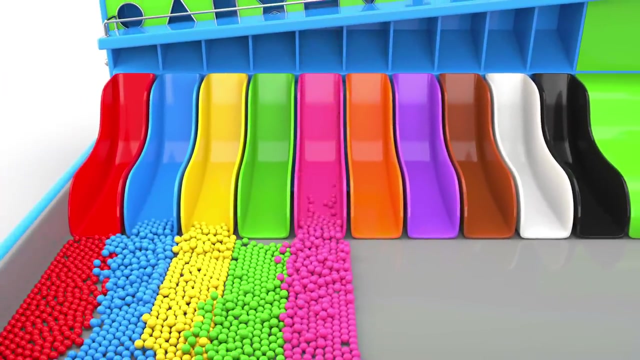 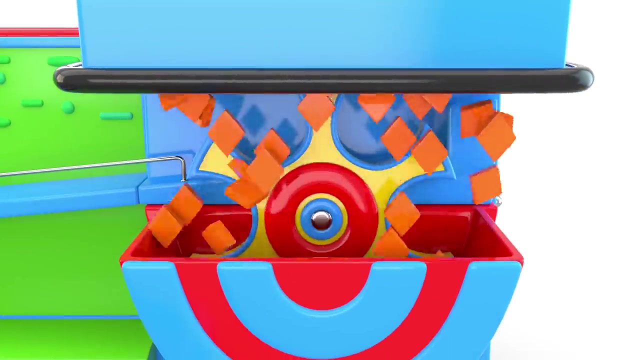 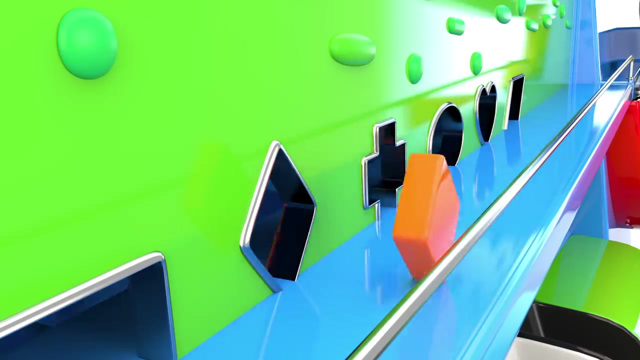 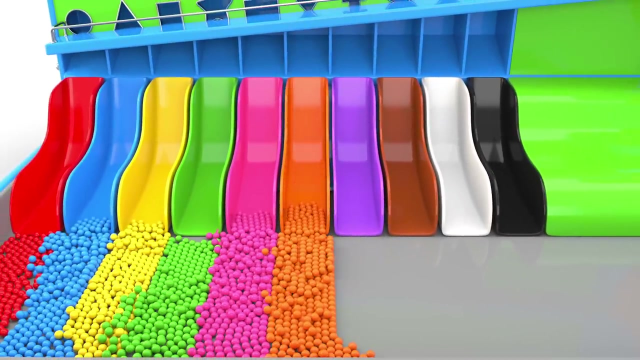 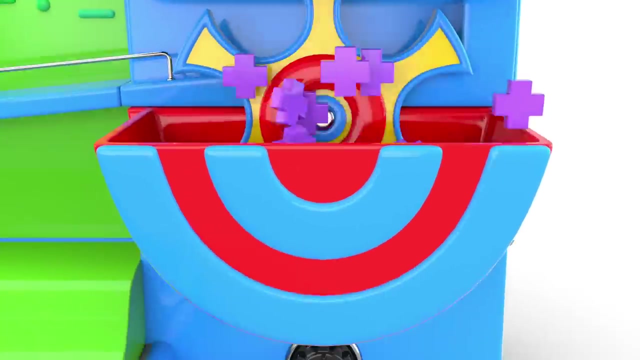 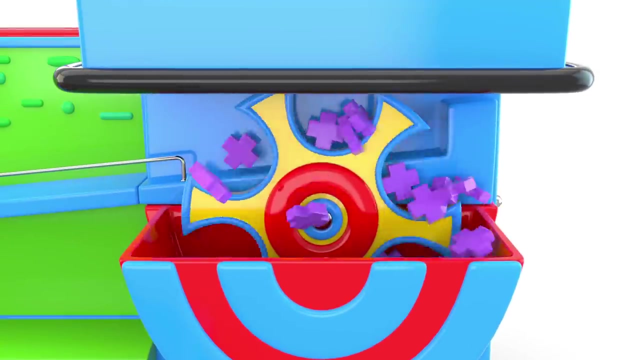 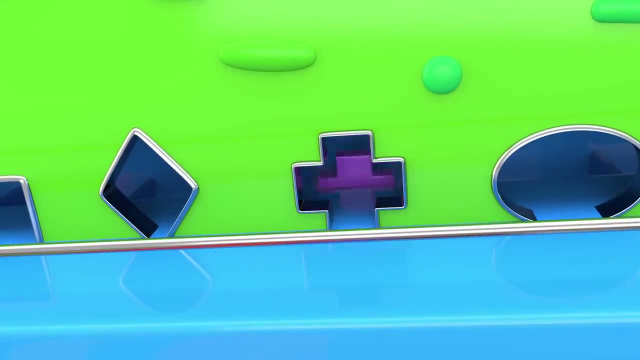 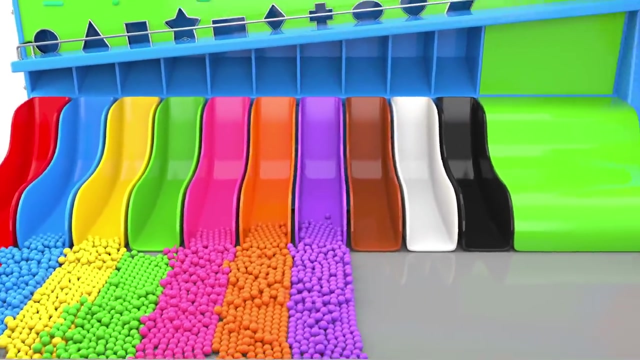 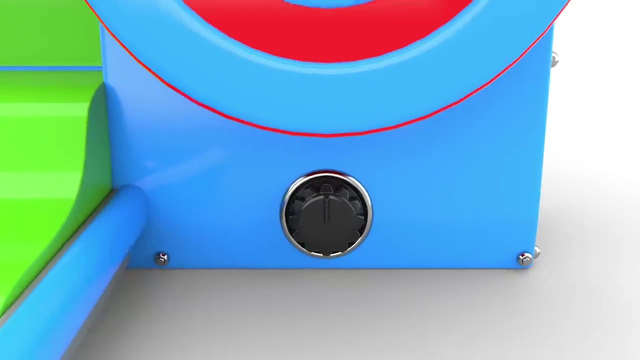 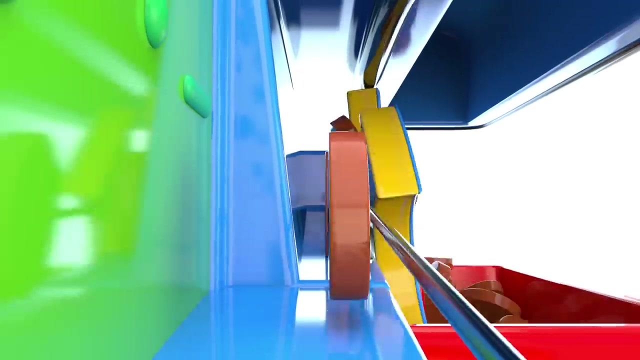 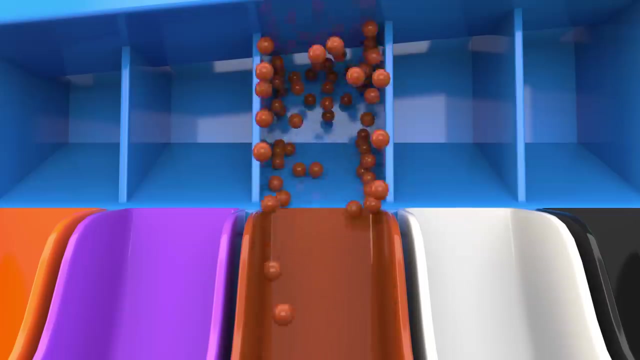 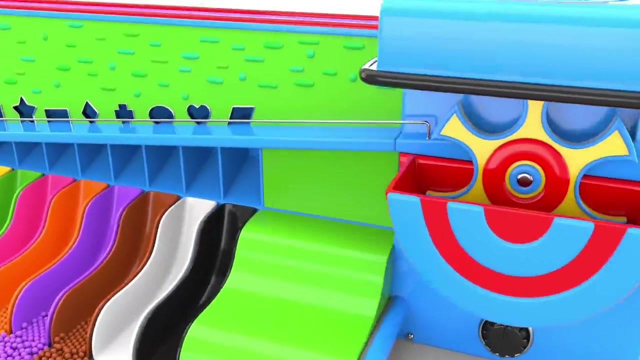 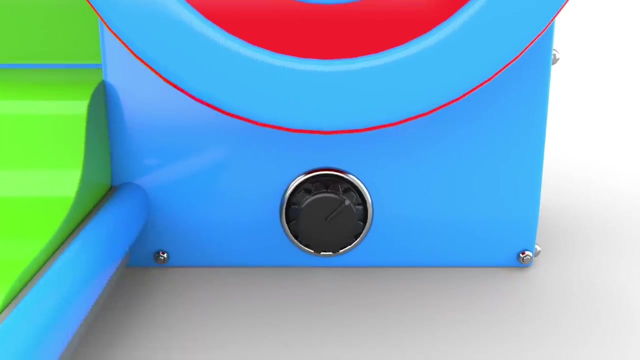 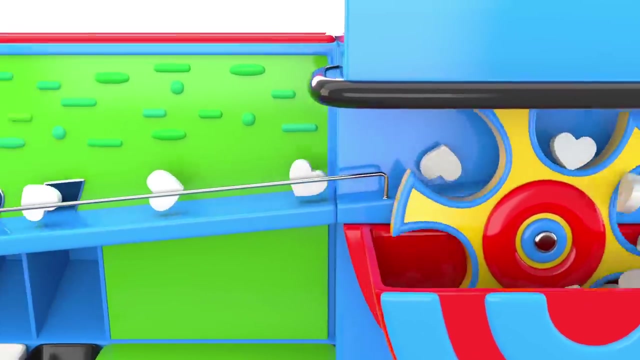 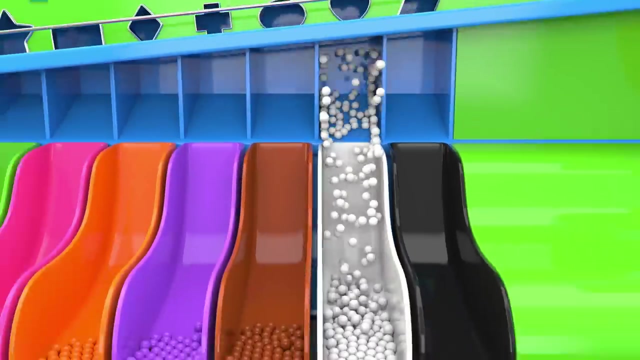 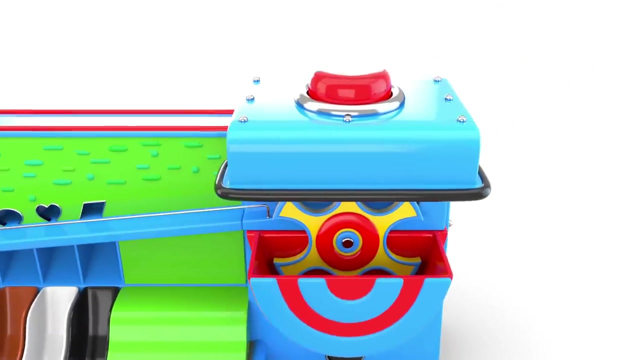 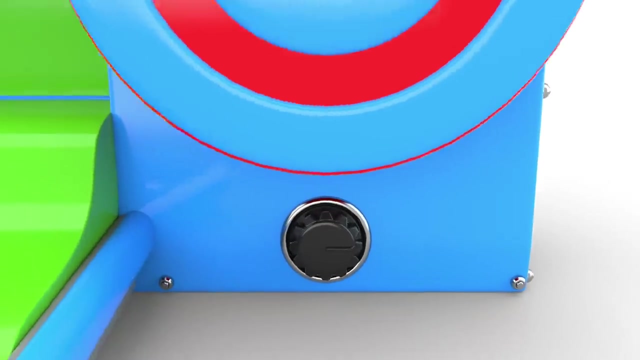 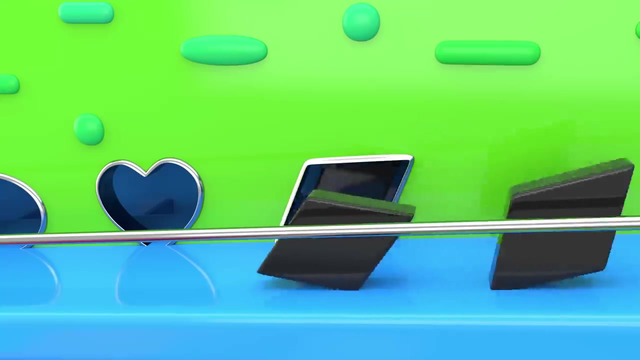 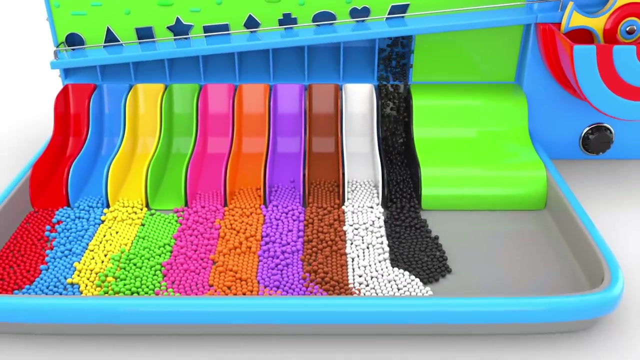 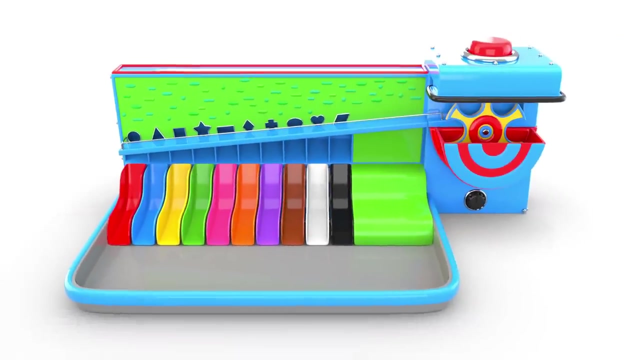 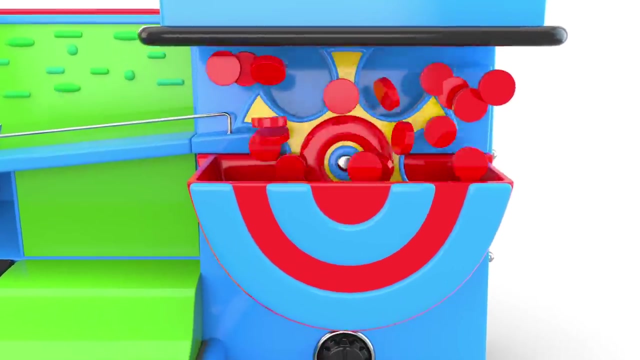 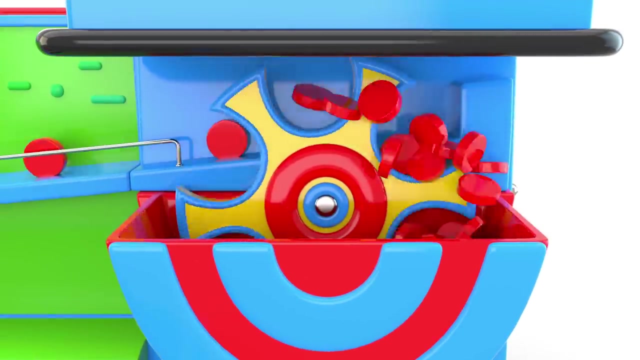 Circle, Rad Triangle, Blue Square, Yellow Star, Green Rectangle. Pink Rhombus, Orange Cross, Purple Oval Oval Oval Oval Rectangle- Rectangle: The Crush, The Crusher. white parallelogram. black parallelogram, parallelogram, parallelogram.